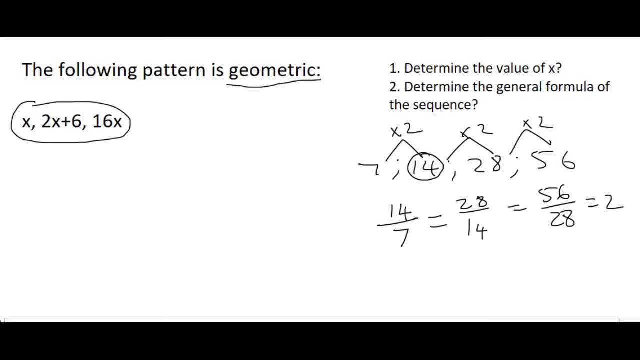 there's x's involved. if that's a geometric pattern, then it means that 2x plus 6 over x should be the same as 16x over 2x plus 6.. Can you see that? I've done exactly what we did. 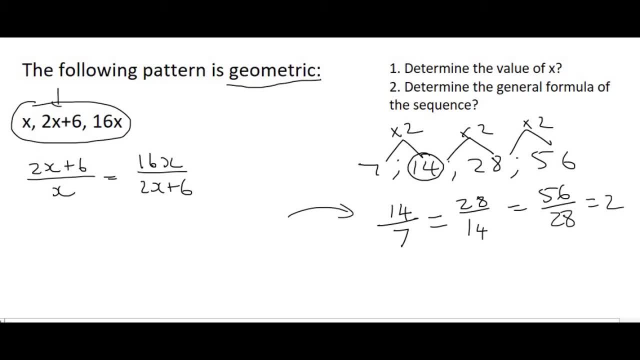 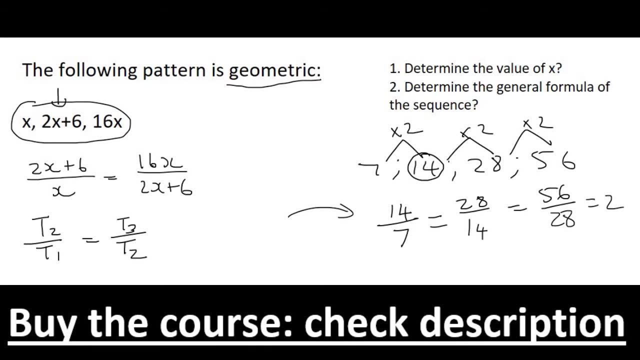 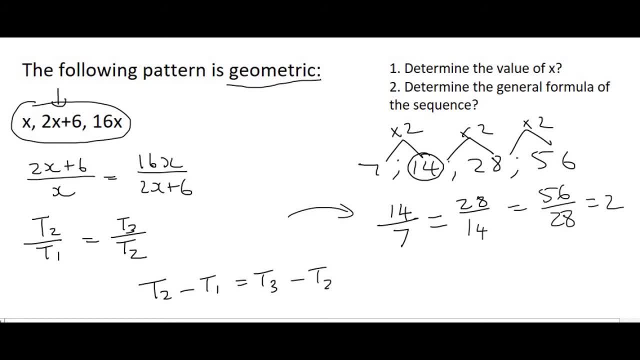 So we're going to do that, So we're going to do that, So we're going to do that, So we're going to do: minus t1 equals to t3 minus t2.. But that only works with arithmetic patterns where the difference is the same. But now the ratio is the same, So we do this instead. And so now, whenever 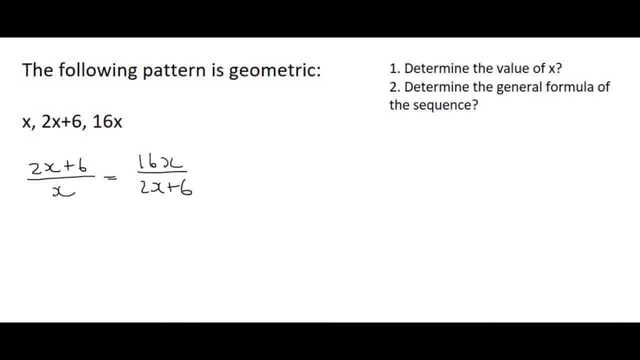 you are faced with a situation like this in maths. all you do is you do cross multiplication. So that goes there and that goes up there. So what we end up with is 2x plus 6 times by 2x plus 6. 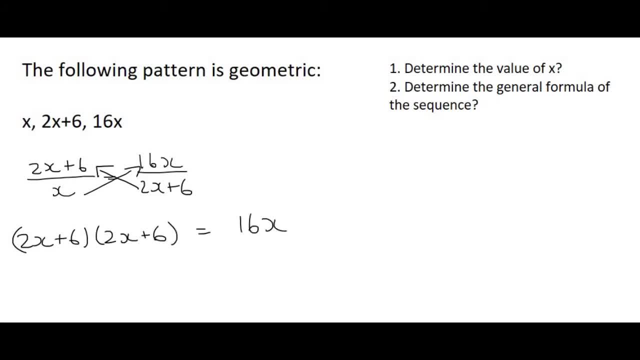 equals. on the right hand side, we have 16x times by x. You see, so I've just done cross multiplication, And so now what you would go and do is you would go multiply all of this together, And so we end up with that, Just. 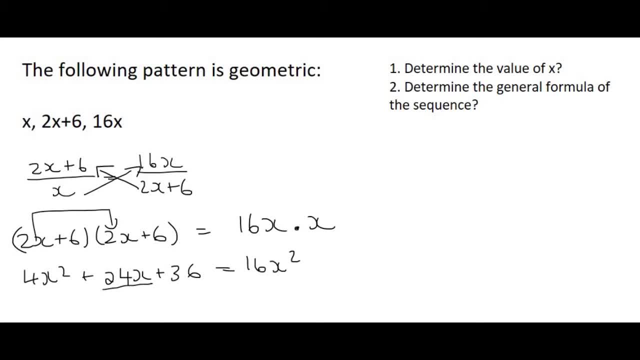 note this: 24x. I did it all in one step, But if you multiply it out the long way, you'd get 12x plus 12x, And then that just simplifies to 24x. Now we've got an arithmetic pattern over here, So 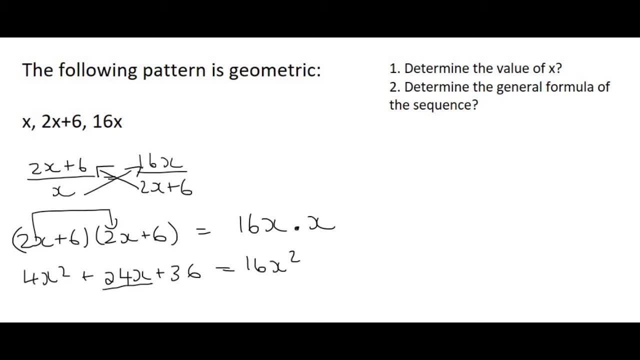 not an arithmetic, a quadratic equation, And so I'm going to take everything to the right hand side, because this number is bigger. You don't have to do it like this. So I'm going to have 0 left on the right, I mean on the left. 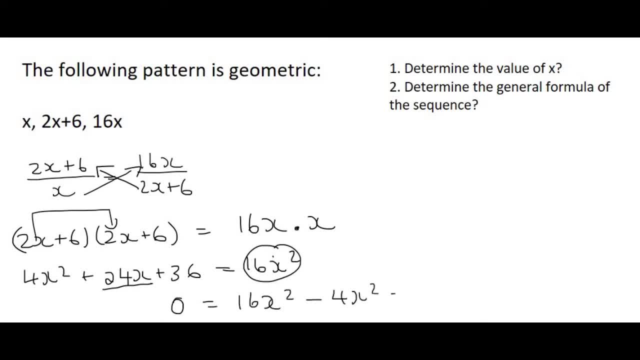 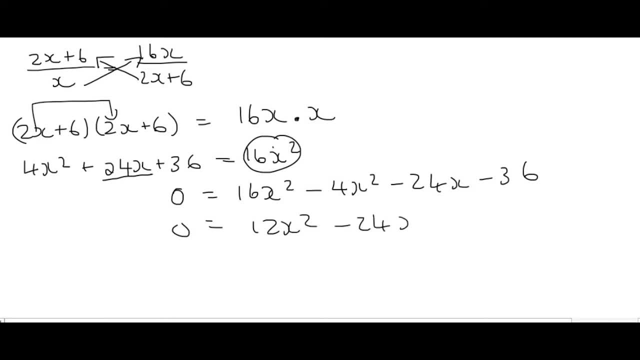 And on the right hand side, we're going to have 16x squared minus 4x squared minus 24x minus 36.. And so that's going to give us 12x squared minus 24x minus 36.. There's a common factor there of 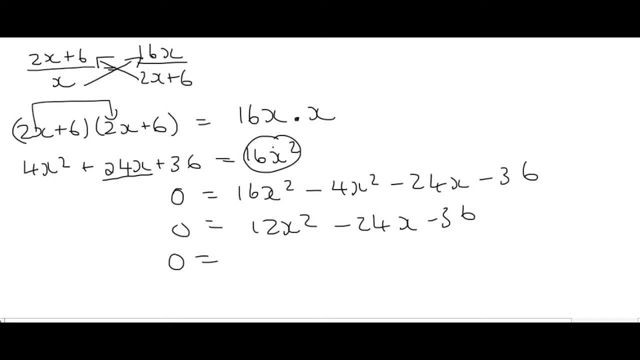 12.. So I'm just going to get rid of that completely Because, remember, when you have a 0 on the other side, you can just get rid of your common denominator or common factor, And that common factor is sorry if I said denominator in this. 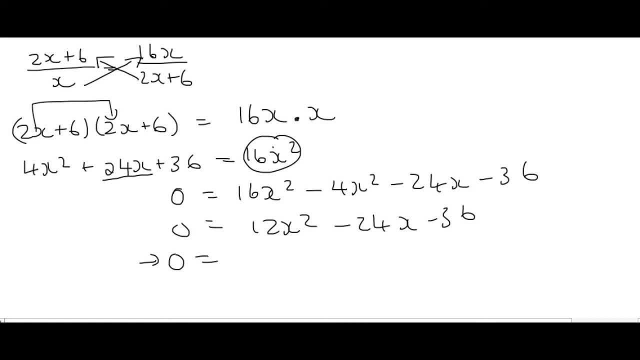 like 30 seconds ago, I'm in Common factor, So you take out a 12., And so that's going to leave you with x squared minus 2x minus 3.. You then get rid of the 12., And so you end up with 0 equals to. 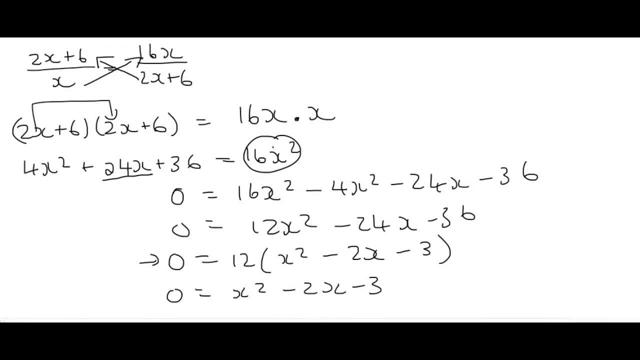 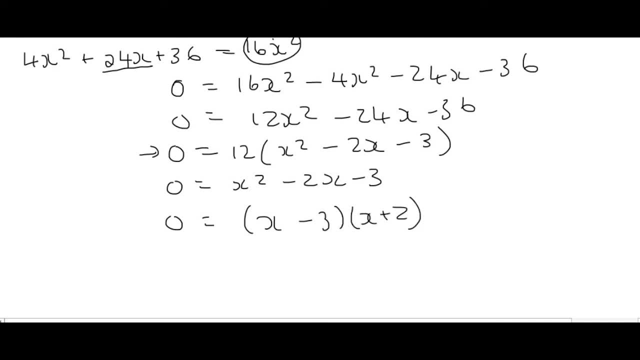 x squared minus 2x minus 3.. Here you could solve this using the quadratic formula, Or you could realize that it's a fairly easy trinomial, And so that's going to give us something like that. So this will be a 1.. And so our two answers are going to be x equals to 3 or x equals to. 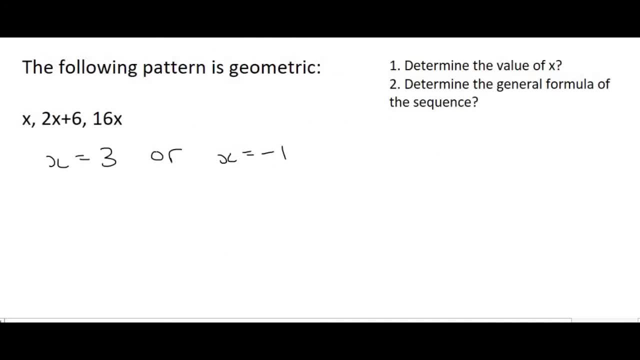 negative 1.. Ah, so we have two answers. Then number two says: determine the general formula. Well, we know that an arithmetic sequence has the general formula like this, But first we should fill in the values of x. So in this video I'm only going to do this one, But in a 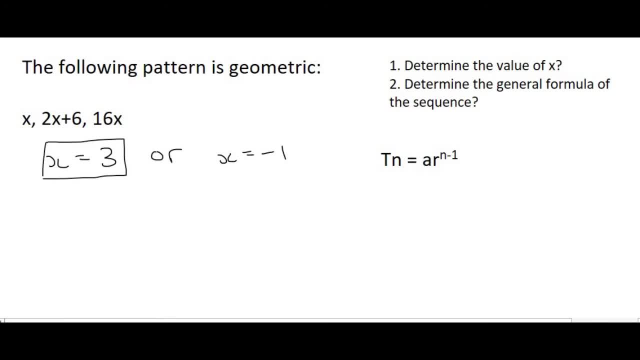 test, you would have to do the same. You'd have to do this question for both. OK, so I'm just going to do the three, just to save you guys some time. So x is 3. So I'm going to fill in 3.. Then, if x is: 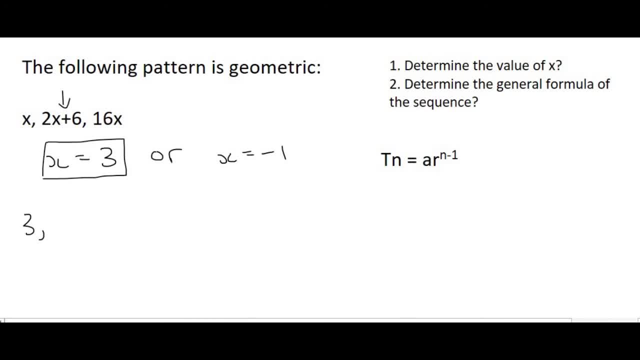 3,. well, that's going to be 2x squared minus 3.. So I'm going to fill in 3.. So I'm going to fill in 3.. 2 times 3,, which is 6,, plus 6,, which is 12.. And then 16 times 3 is 48.. And so there's our 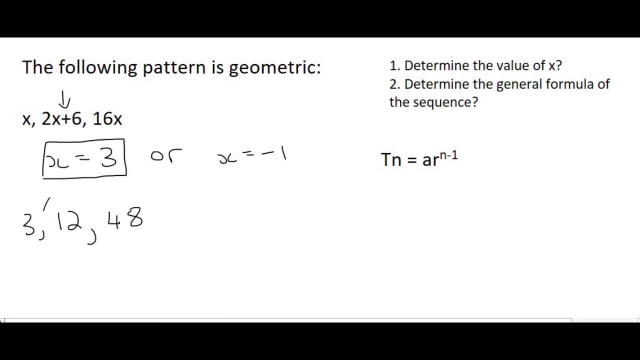 geometric sequence If we have. let's just check it out. Well, to get from 3 to 12, you would times by 4.. And to get from 12 to 48,, you times by 4.. So it does work. And then, 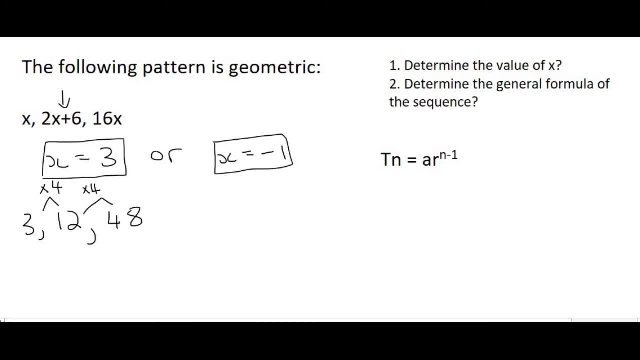 of course you could do this one for minus 1.. But then that becomes a totally new question. You would have to do it two separate questions. So determine the general formula. Remember when we're looking at arithmetic, general just means. 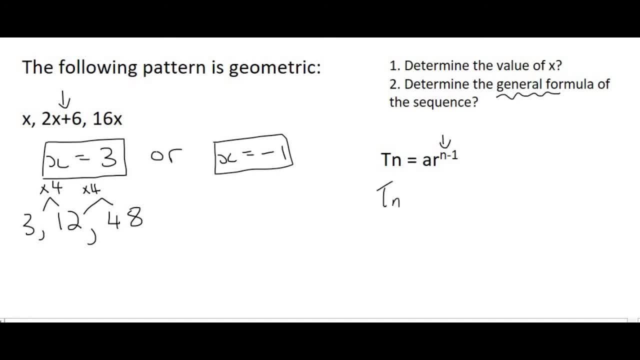 we don't know what the position is. We're just going to fill in whatever we have, So we'll just go. tn equals to a. Well, a is always term number 1, which is 3.. r- r is the number that. 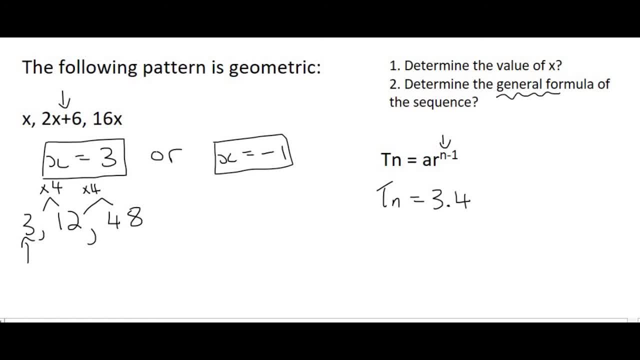 you have to multiply to get to the next term, So that'll be 4.. And then n minus 1, we don't know, So we just leave it like that. Now, as I said in a previous video, the most common mistake is that.